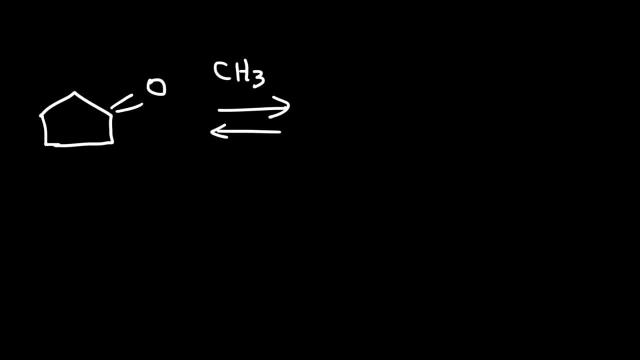 ahead and predict the major product if it reacts with methanol under acidic conditions. So this can go all the way to an acetyl. Let's say if we use excess methanol So we can get two OR groups, And then if we react with H3O plus we can. 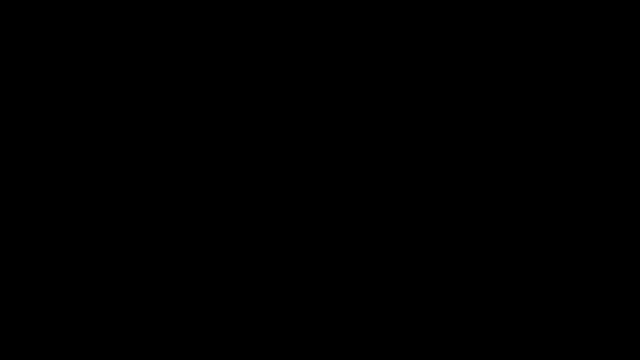 regenerate the original methanol. Now let's go over the mechanism for the formation of an acetyl group. So because the reaction occurs under acidic conditions, the first step is protonation. So once we add the hydrogen to the oxygen atom, this group becomes more. 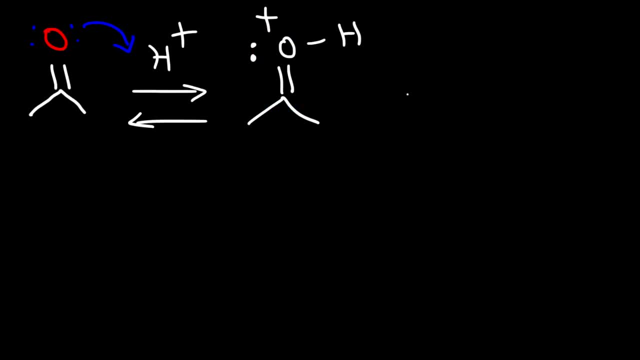 electrophilic, more susceptible to nucleotides. And then the second step is the nucleophilic attack by the methanol molecule, And so the oxygen atom of methanol is attracted to the partially positive carbonyl carbon, And so the methanol attacks there. 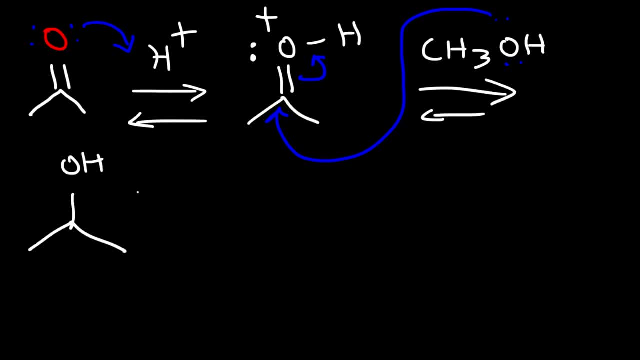 Now the double bond is going to break, so we're going to get an OH group And here we have an oxygen attached to a hydrogen and a methyl group, And now that oxygen has a positive charge, Now what we need to do at this point is we need to get rid of this hydrogen atom. 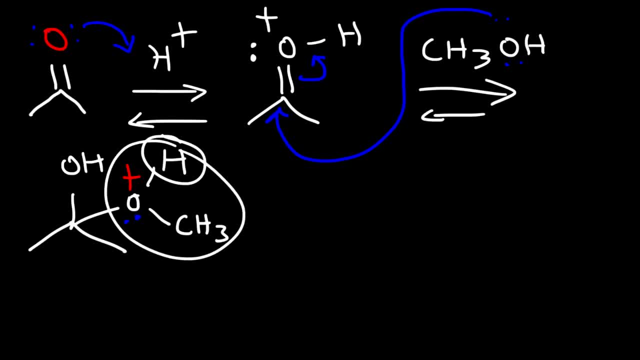 Because right now this group is a good leaving group. Anytime oxygen has three bonds it's a good leaving group, And so this OH group. what it could do is take a lone pair, form a double bond and just kick this group out, giving us this compound. 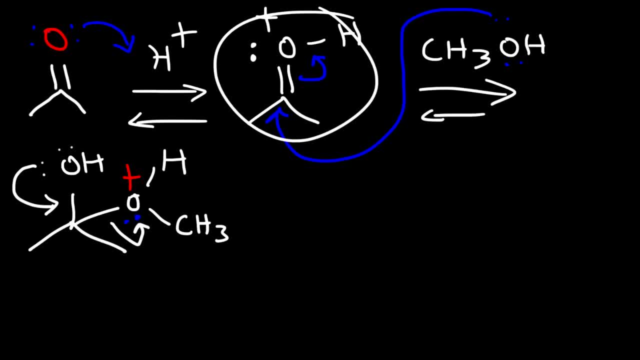 So that's going to take us a step back, which we don't want to go in that direction, And so what we need to do is get rid of the hydrogen. So let's use another methanol molecule to act as a weak base. 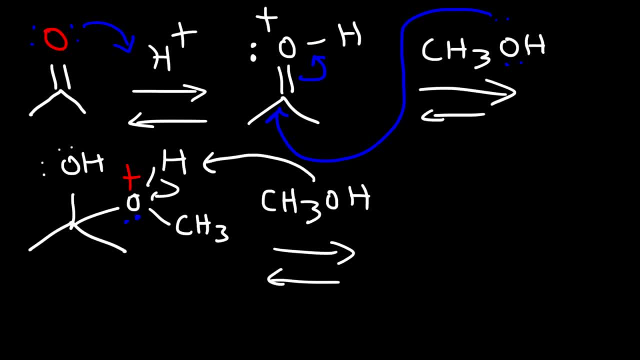 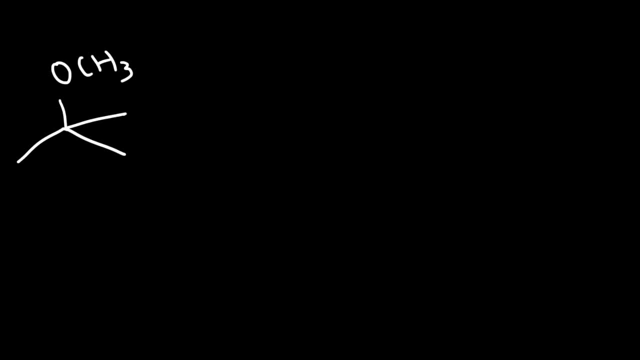 And so it's going to take away this hydrogen for us, which is what we want it to do, And so now we have an OR group and an OH group. So now the methanol that took the hydrogen away. It's now Okay. 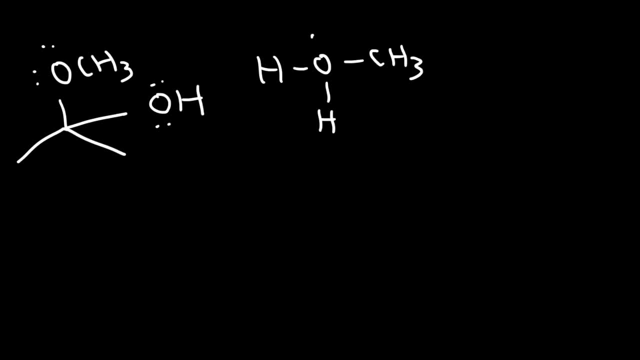 protonated, And so what I'm going to do is take a hydrogen from that protonated alcohol and transfer it to the OH group. We want the OH group to be a good leaving group because we need to get rid of it, And so let's take a lone pair from oxygen from the OCH3 group, form a. 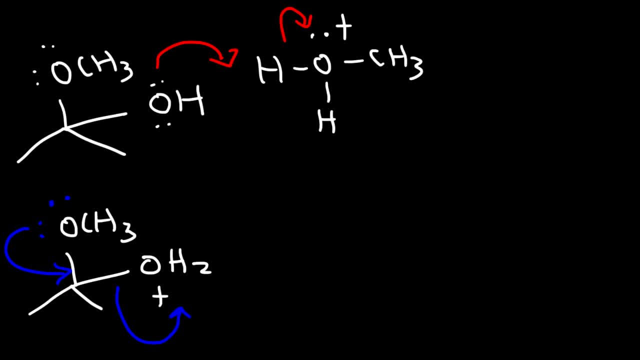 pi bond and let's kick out water, So this arrow should be pointing towards the oxygen atom. It didn't look like it was doing that before, And so this is what we now have. So what do you think the next thing is going to? 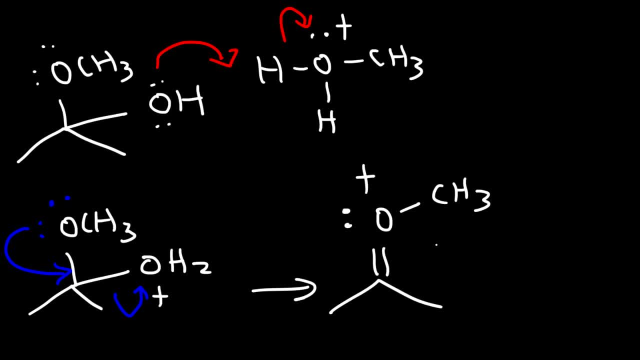 be. What's our next step here? So right now we have this group which is highly electrical. So right now we have this group which is highly electrical Because if we draw the resonance structure, we can put a positive charge on the carbonyl carbon. 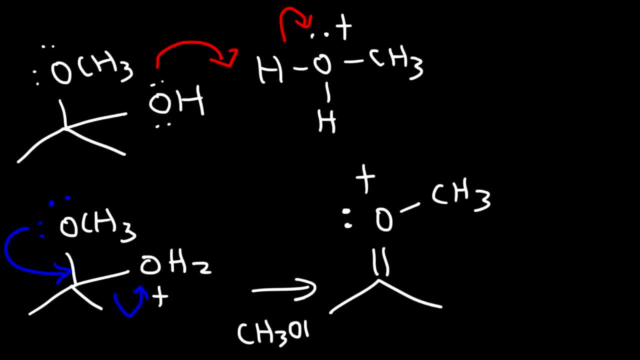 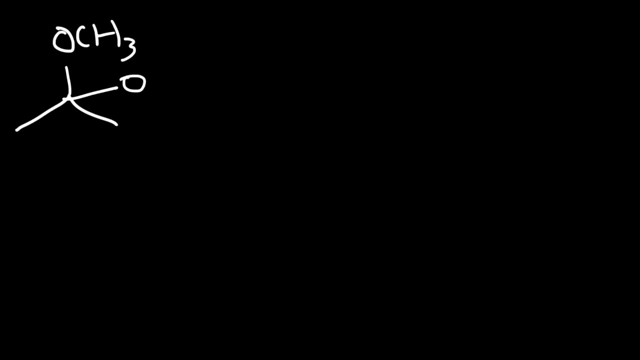 So what we're going to do is take another methanol molecule and react it with the carbonyl carbon, So it's going to attack here, breaking this pi bond. So this is what we now have. In addition to the OCH3 group, we have another OCH3. 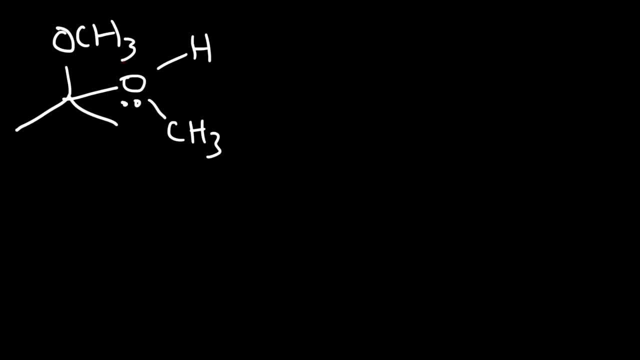 group, but with a hydrogen atom attached to it, And so the last step in this mechanism is deprotonation. So let's use another methanol molecule to get rid of that hydrogen, And so we're going to have a hydrogen atom, And so we're going to have two OCH3 groups, And so this is the mechanism for. 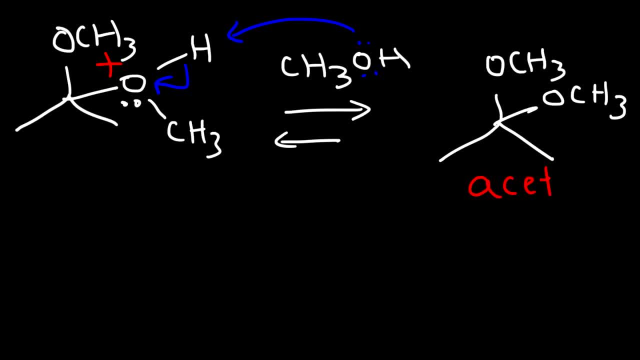 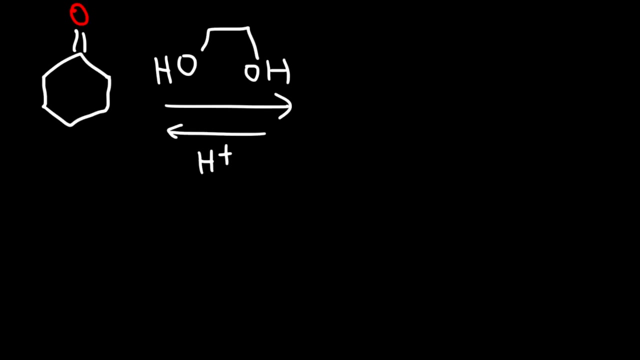 the formation of the acetyl functional group. Now let's go over the next reaction. So let's say, if we have cyclohexanone and we wish to react it with ethylene glycol, What's going to happen Now? in the previous examples we saw that when mixing an aldehyde or a ketone with 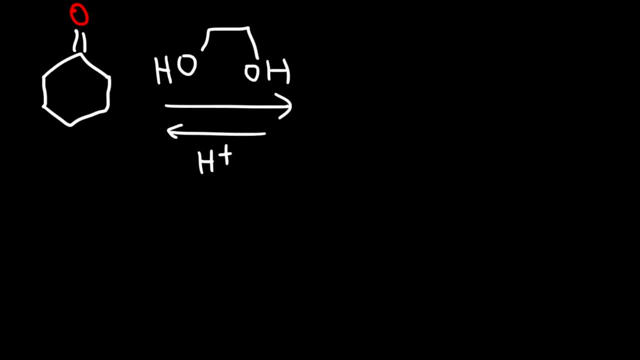 one alcohol molecule, we got a hemiacetyl. But when mixing it with two alcohol molecules, we got an acetyl. Well, ethylene glycol is one molecule but with two alcohol functional groups. So what we're going to get is the acetyl but a. 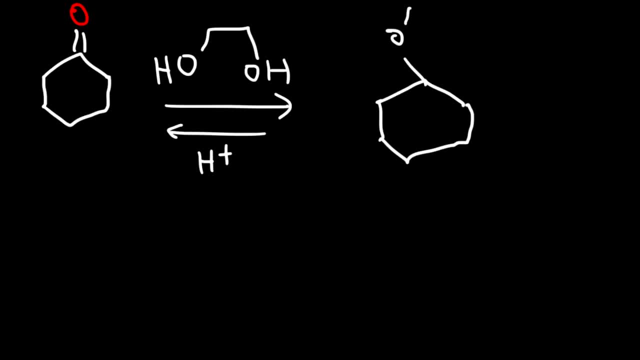 cyclic acetyl And it's going to look like this. So we have two OR groups connected to each other, And this reaction is useful as a protecting group. Now we can remove the protecting group by reacting it with H3O+, And so that is going to regenerate the ketone. So here is an. 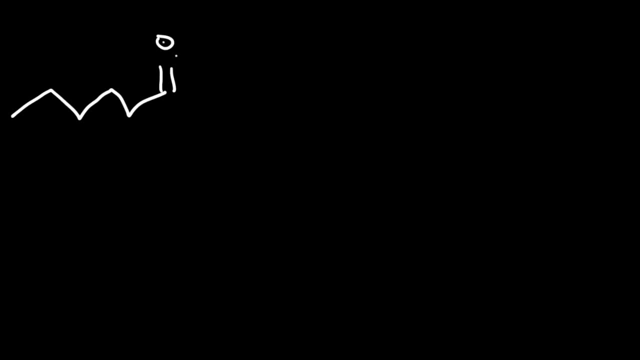 example that will illustrate the use of the protecting group. So here we have a molecule that contains a ketone and an ester functional group. How can we use a protecting group in a way that we can reduce the ester to an alcohol but not reduce the ketone to an alcohol? 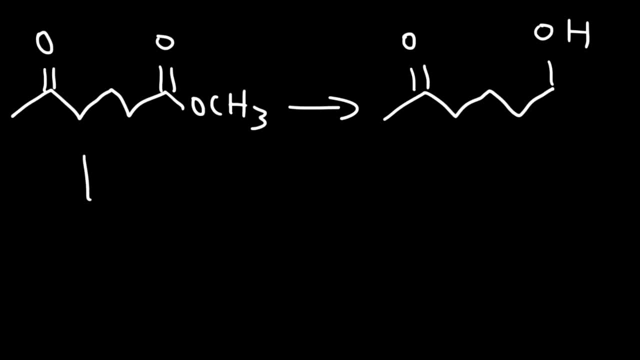 Now, if we use, for instance, sodium borohydride, Sodium borohydride can reduce the ketone to an alcohol, but it can't reduce the ester, And so we're going to get this product, Which is what we don't want. 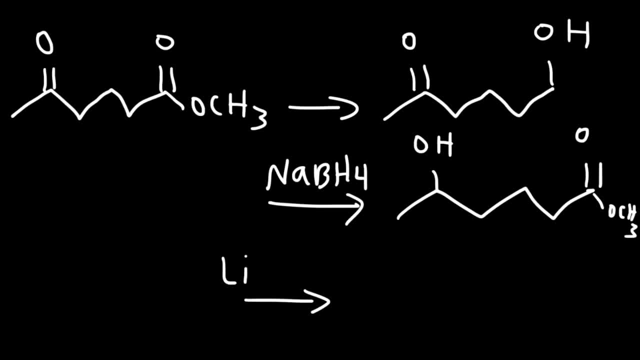 now, if we use a lithium aluminum hydride, it will reduce everything. it can reduce the ester into an alcohol, but it will also reduce the ketone to an alcohol. now we don't want to use sodium borohydride because we need to reduce the ester to. 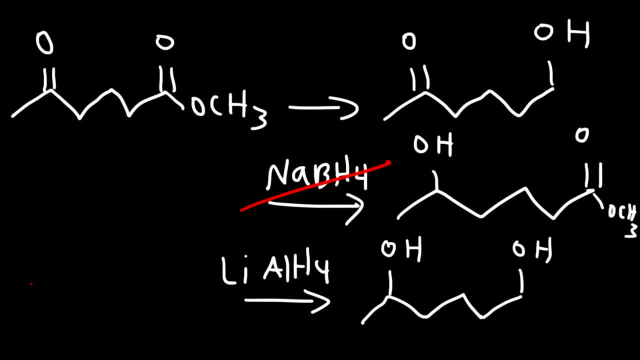 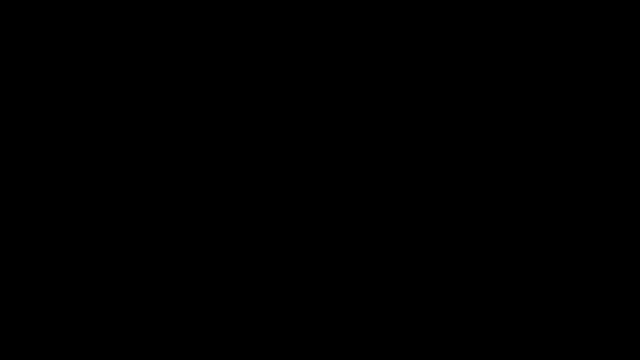 an alcohol and sodium borohydride can't do that, so we could eliminate that option. now we want to use lithium aluminum hydride because it can reduce the ester to an alcohol. however, we don't want it to reduce the ketone, so what should we do? it's important to understand that ketones are more.